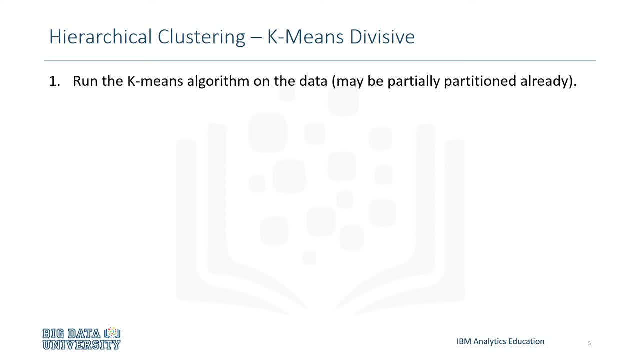 The first step is to run the k-means algorithm on the original dataset. This dataset may already be partially partitioned or may just be one large cluster. We choose a value of k, which is how many subsets we want to break the cluster into. So C3,, for example, will 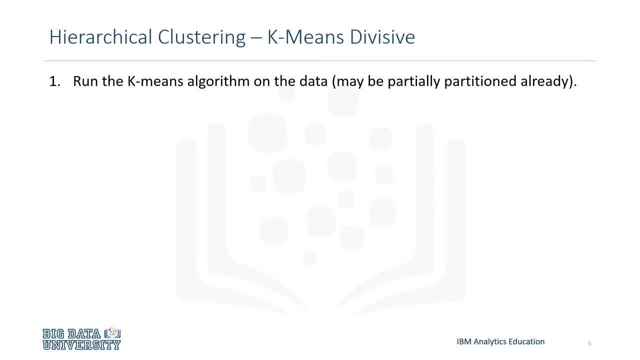 be quantized with a number of não. Now we can use that n as well. Now let's take a look at some undoing operations. Let's try these. Push the button, ideally, while guilt-free running. Push the button until the data points are in the赤 box with the stereotypical arquitectural. 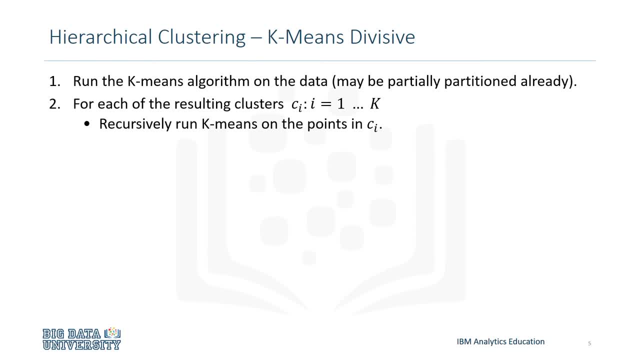 and 용-iempo going to the走线box. For each variable of our algorithm, we can route data points to the k-means algorithm. The way this совершic ls, to my understanding, is numeric. The first result is this: 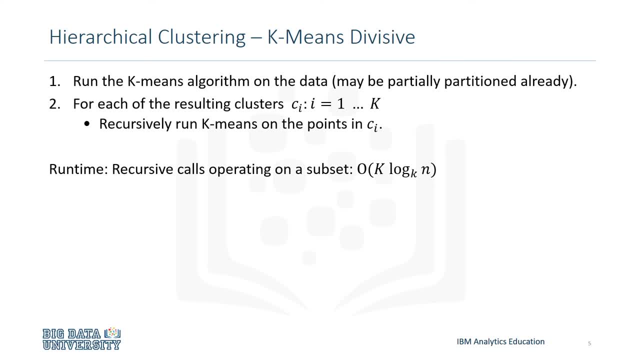 When we run this recursively, we run, we continuously run- cases of k back and forth, That categories are read by a variable setup with more places, where n is the number of data points and k is the number of clusters you produce from each cluster in every iteration. 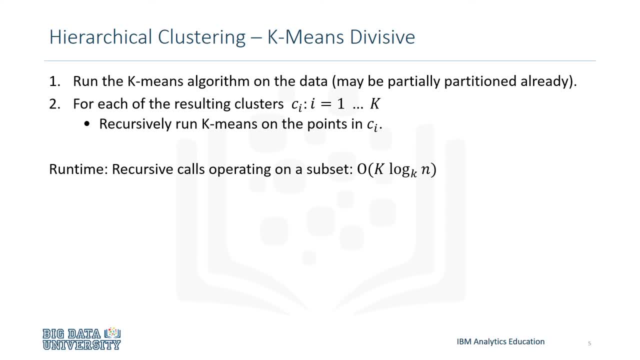 So, for example, k equals 2 would split a cluster into two clusters, then each of those clusters would be split into two more clusters, totaling four clusters, and so on. Note that whenever a cluster is split into different subsets, the clusters are never merged again. 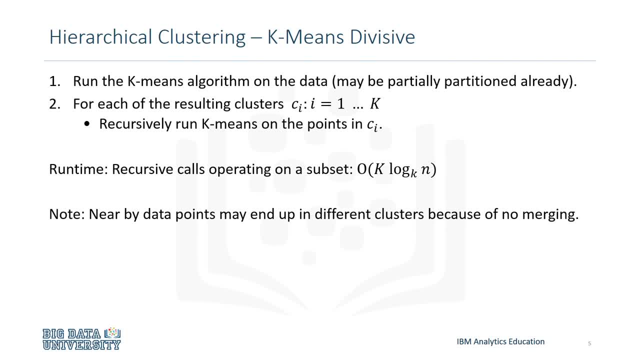 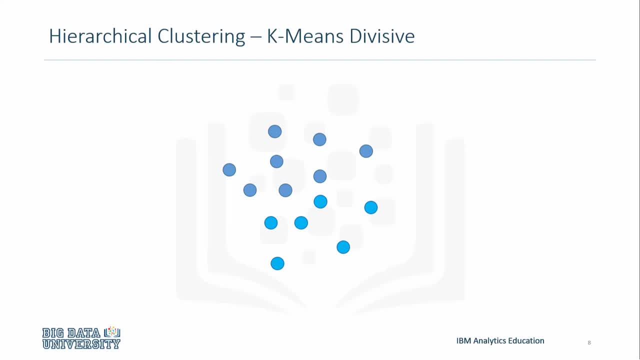 Again, the k-means algorithm only runs in each specific subset of data that it's working with. Here's a quick example of k-means hierarchical divisive clustering. Let's say we start with a data set that looks like this: We'll also be working with k equals 2.. 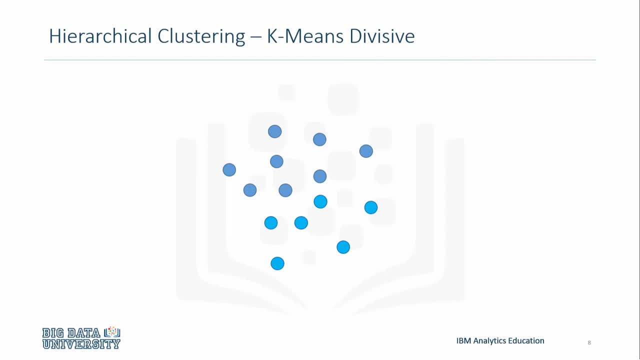 So when we run k-means on these two clusters, we get something that looks like this: Now we have two clusters, one blue and one red- k-means 1.. We'll now run recursively on each of these clusters And let's look at one more split. 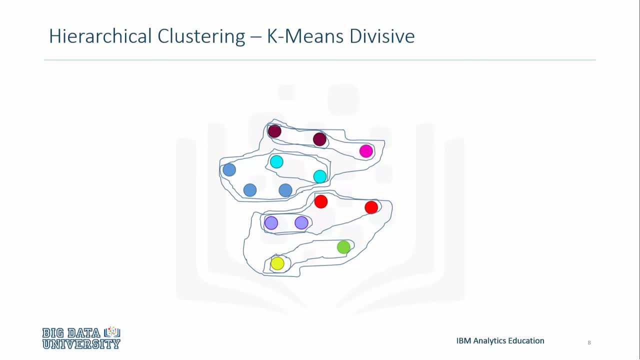 As previously stated, this would simply continue until each point was in a cluster of its own. Thanks for watching.